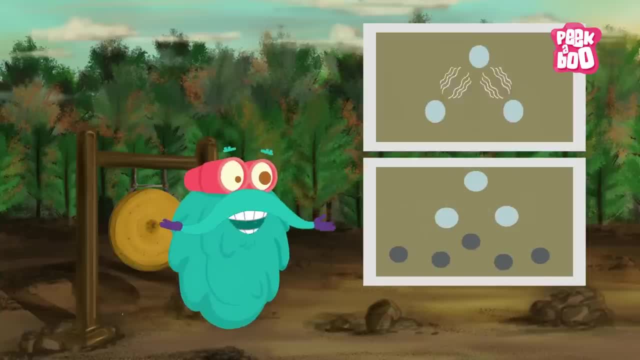 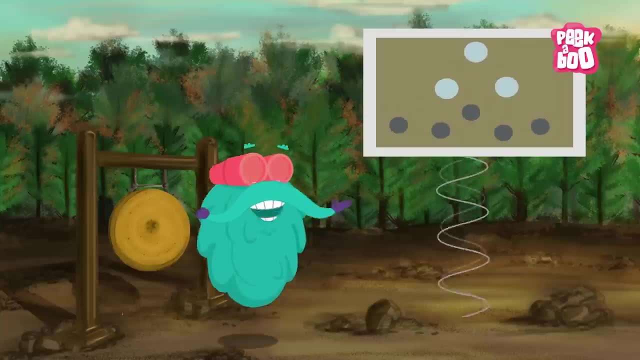 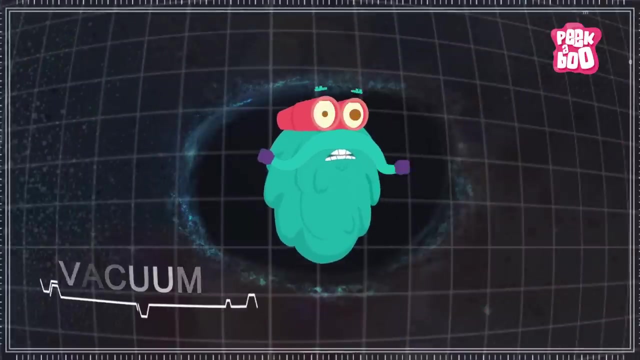 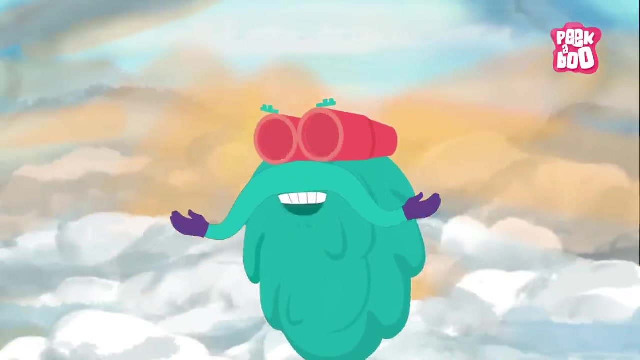 Which in turn causes the other molecules around them to vibrate. And these vibrations from one molecule to the other other help sound to travel. You couldn't hear me right? Well, because I was in vacuum, In spaces where there is just vacuum and no matter. 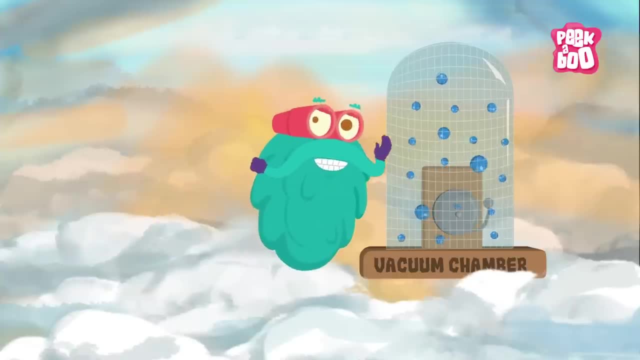 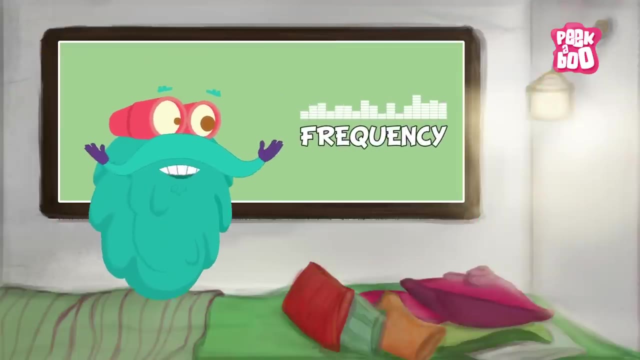 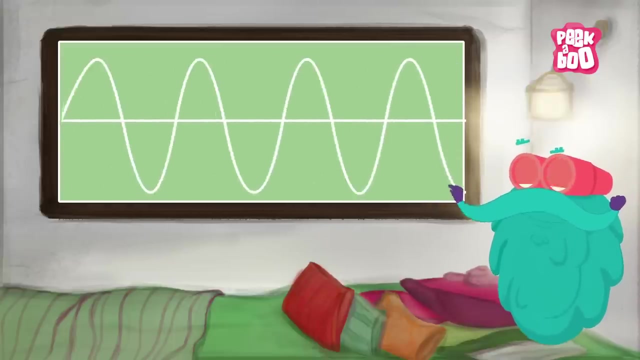 Sound will not travel because there won't be any molecules to vibrate Freak out. Frequency is an important measure of sound. When there are more number of sound waves passing through a fixed place at a given time, it means that the frequency is high. 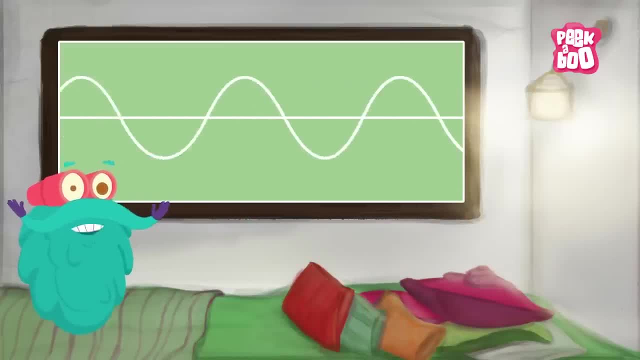 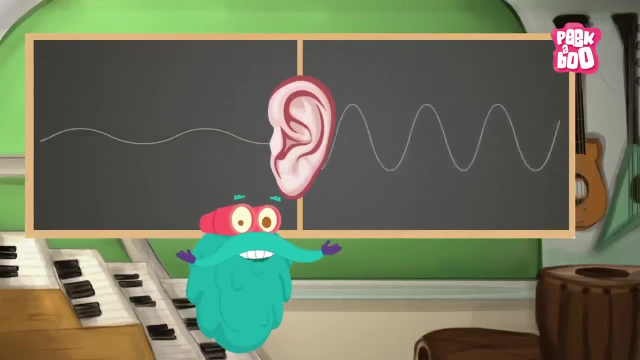 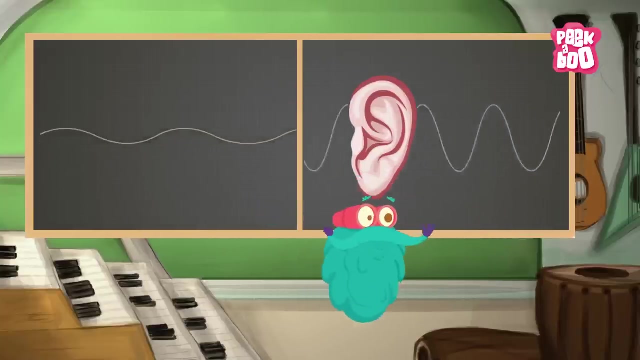 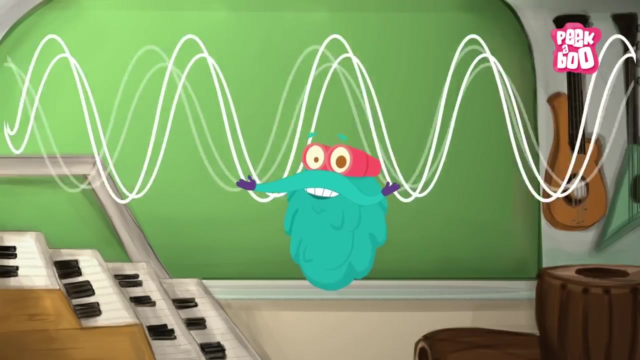 When the number of waves become less, we hear low frequency sound waves. The human ear is capable of detecting frequencies between 20 Hz to 20,000 Hz. The frequency above or below that is inaudible to the human ear. Higher frequency sound waves will give us a higher pitch. 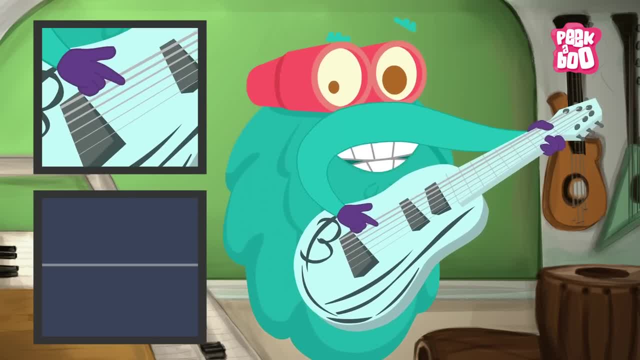 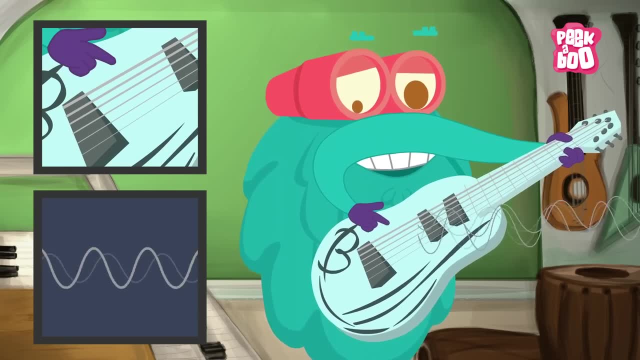 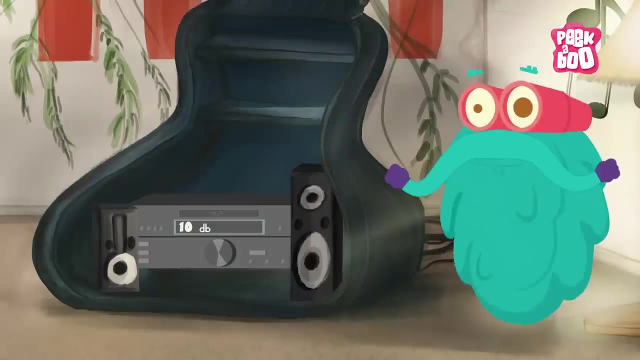 Hmm, take a guitar and play the heavier string. Hearing the buzz? Now play the thinner string. Isn't there a difference in sound? Well, that's the difference in pitch. The loudness of sound is measured in volume. 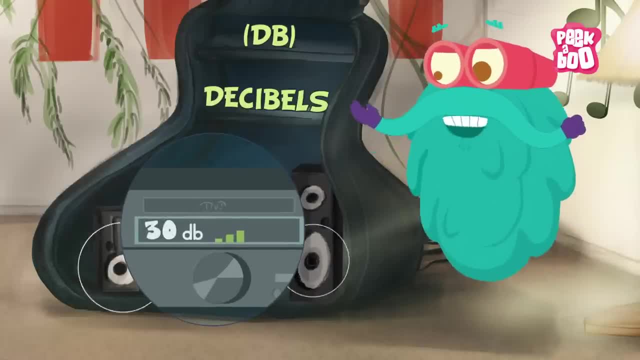 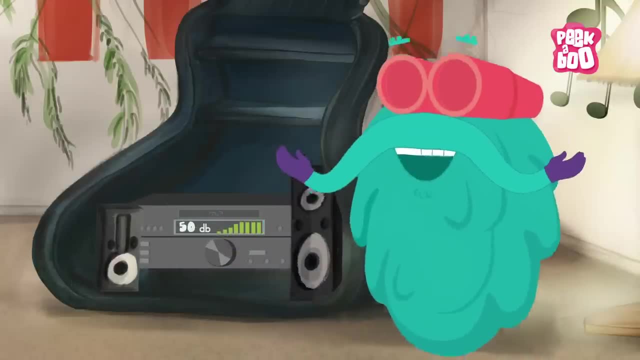 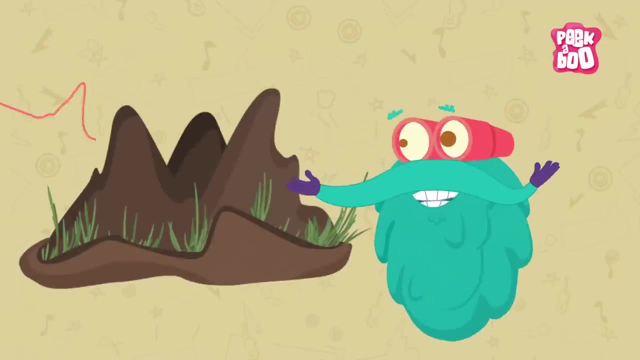 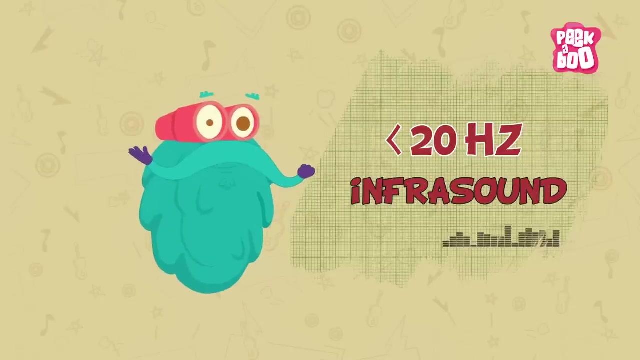 And to quantify volume we use decibels. Here is an example of volume. Can you hear me now? Trivia time? Sound waves can bend around corners and obstacles. Any sound with a frequency below 20 Hz is called Infrasound. 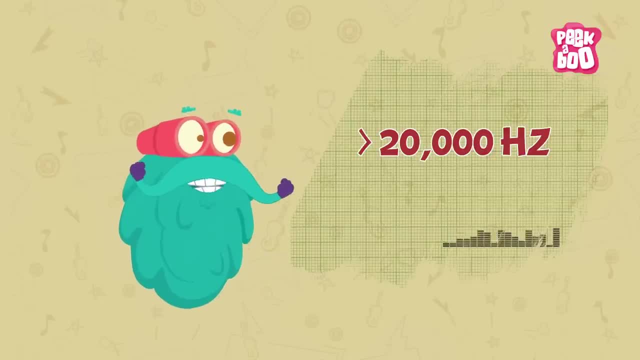 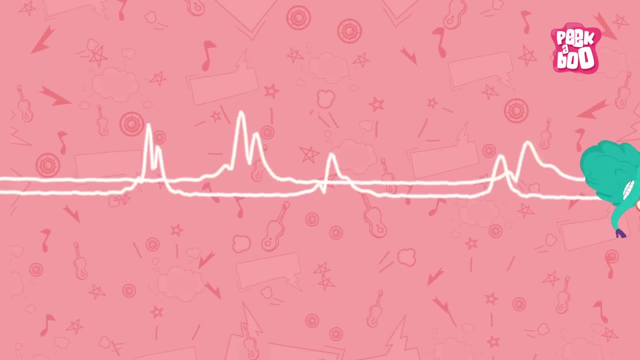 And any sound with a frequency below 20 Hz is known as Ultrasound. So this is me zooming out. Tune in next time for more fun facts.